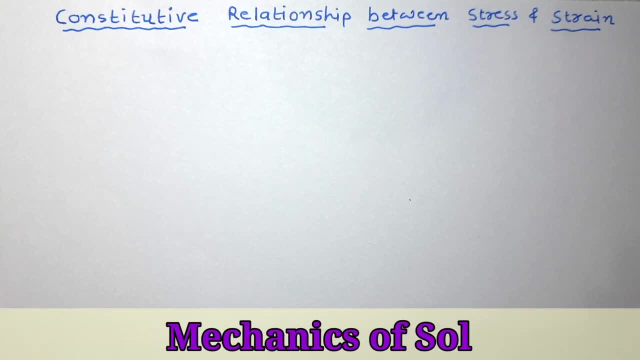 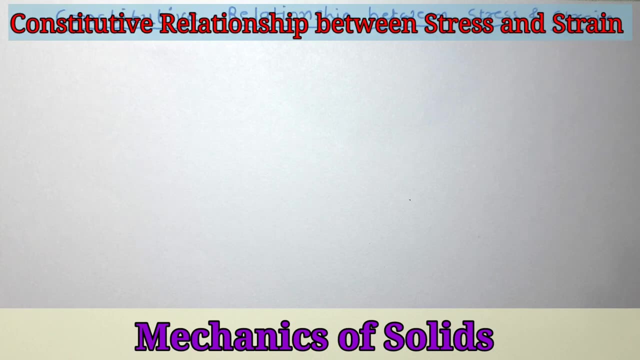 Welcome to the lecture series of Mechanics of Solids. In today's lecture we are going to learn the constitutive relationship between stress and strain. Outlines of the session. In this session we are going to learn the constitutive relationship between stress and strain in first, one-dimensional stress. 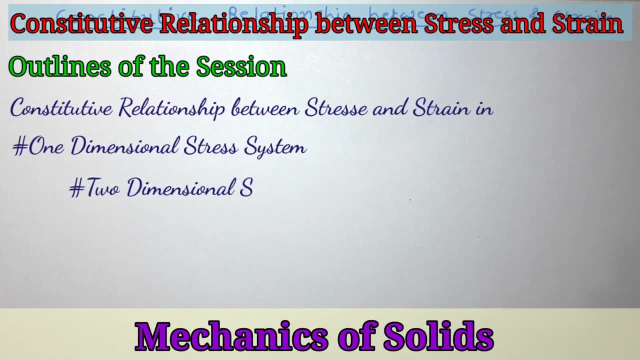 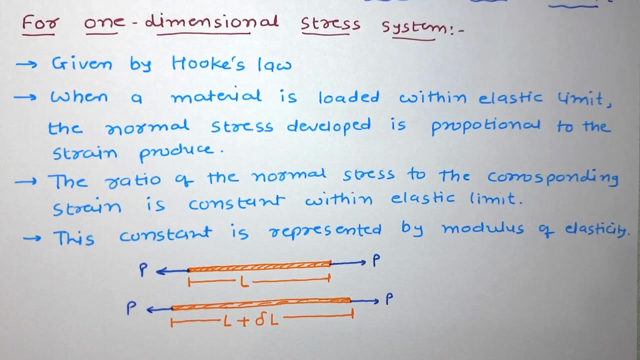 system, Second, two-dimensional stress system and third, for three-dimensional stress system. So let us start with first, That is the constitutive relationship between stress and strain for one-dimensional stress system. so let us try to understand for one-dimensional stress system, here the material which is: 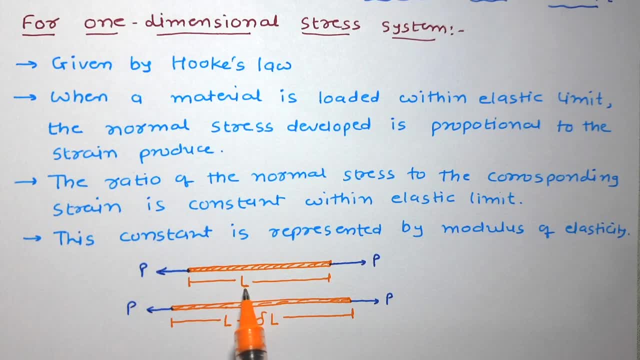 unidimensional means it is having only length. its thickness and width is negligible. so when such material is acted upon by external load P, its length is increases and it reached to L plus Delta L. this load P is applied up to elastic limit. so when such load is applied within elastic 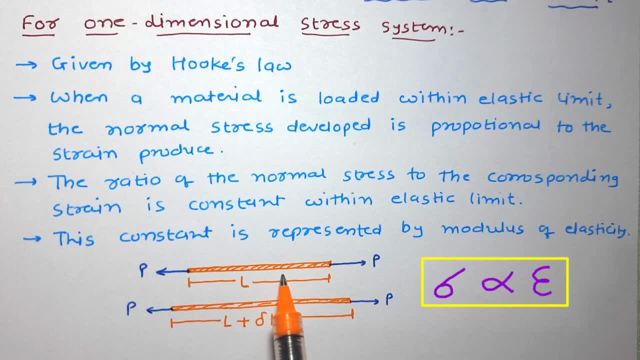 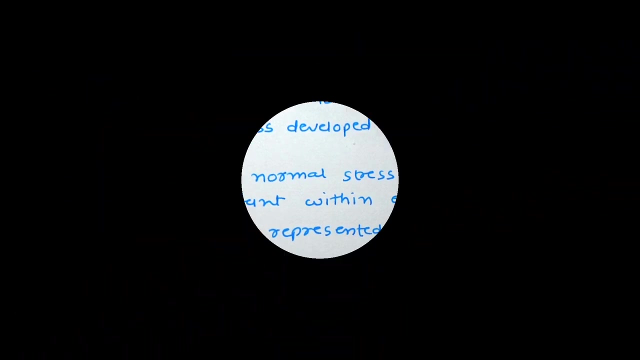 limit. the stress produce in this material is proportional to respective strain produce in the material. so this ratio of normal stress to the corresponding strain is constant within elastic limit. this constant is represented by. we know that it is modulus of elasticity or Young's modulus, and we can. then we denote it by E. so here the ratio of normal stress to corresponding strain. 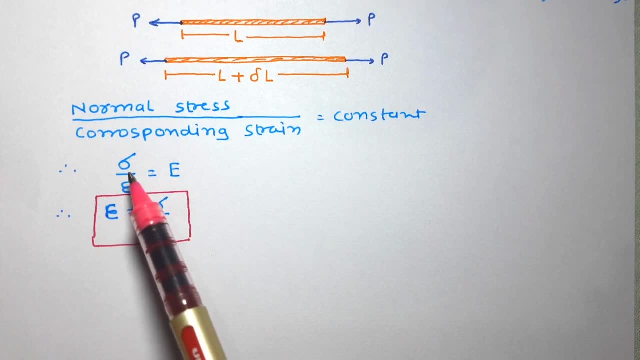 will be constant. so we can write fears that you mean on more stress upon epsilon. that is corresponding strain, that ratio is constant and it is all modulus of elasticity. E or Young's modulus, so we can right in terms of epsilon is equal to sigma upon E. so this is the required relationship between stress and 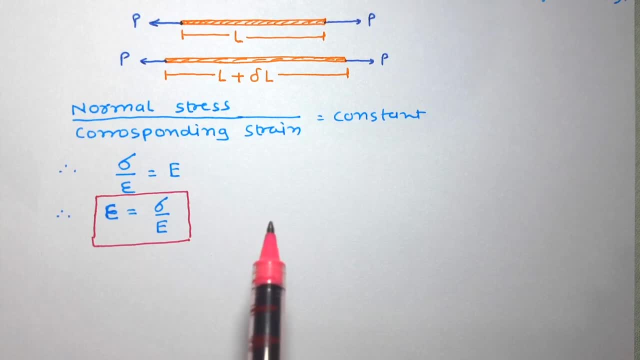 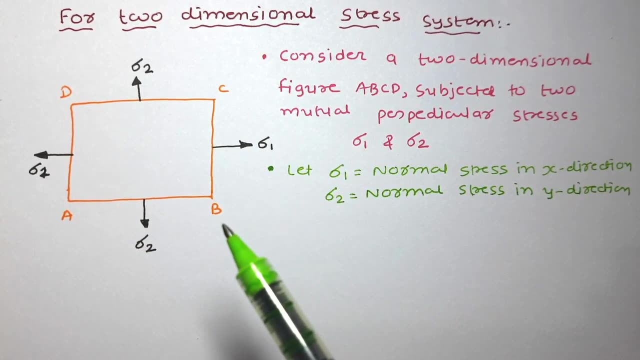 strain in one-dimensional stress system. Well, stress system. so now let us see the constitutive relationship between stress and strain in two-dimensional stress system. consider the figure ABCD, which is two-dimensional figure, and in this figure two stresses which are mutually perpendicular to each other are acting on two mutually faces of this block. let 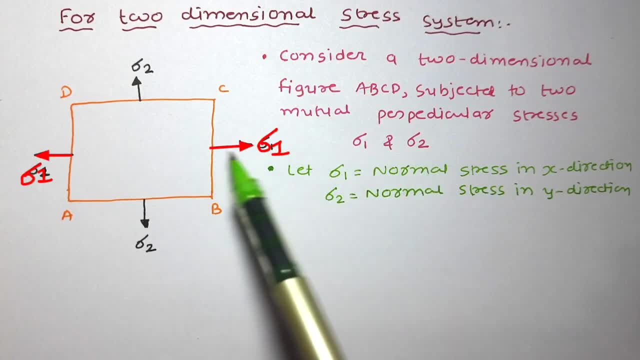 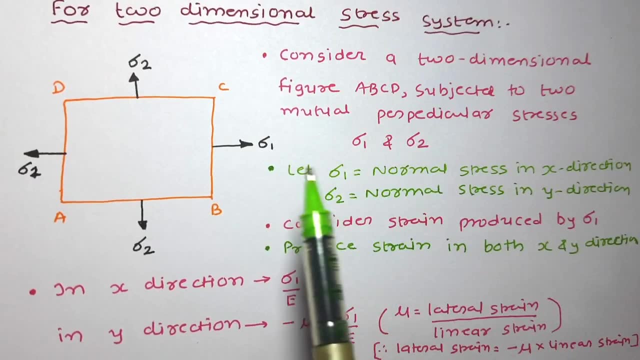 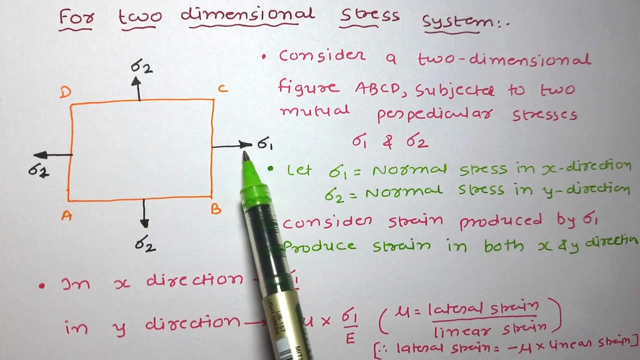 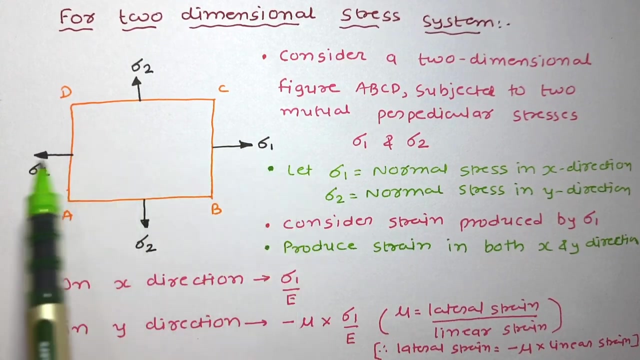 Sigma 1, that is normal stress in X direction, and Sigma 2, that is normal stress in Y direction. so now let us try to understand the strain produced by this stress: Sigma 1, which is acting in X direction, so we can see, and due to this stress, the strain in X direction will be longitudinal strain. 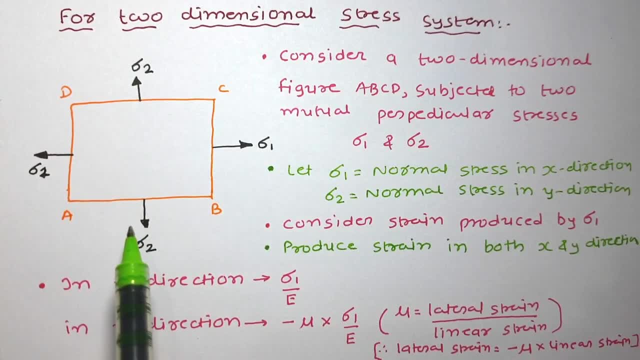 and strain in Y direction. it will be lateral strain, so it will produce strain in both X and Y direction. so stress produced in X direction means in this direction that is equal to Sigma 1 upon E, that is according to hook slope, and in Y direction- we know that Poisson's ratio. 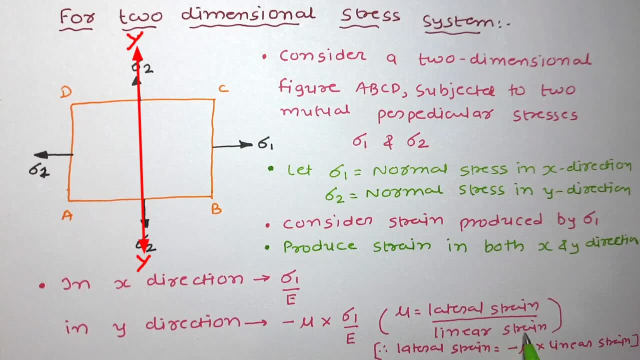 mu is equal to lateral strain upon linear strain. so in this case we can say: lateral strain is equal to mu into linear strain. here we have kept minus because it is in opposite direction to these stress produced in X direction. so stress in y direction that is equal to negative positions ratio into linear strain, right? so we 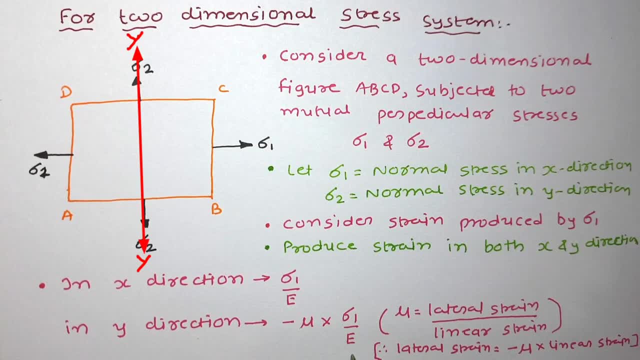 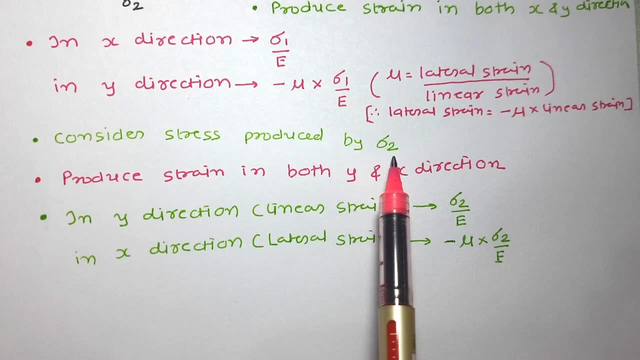 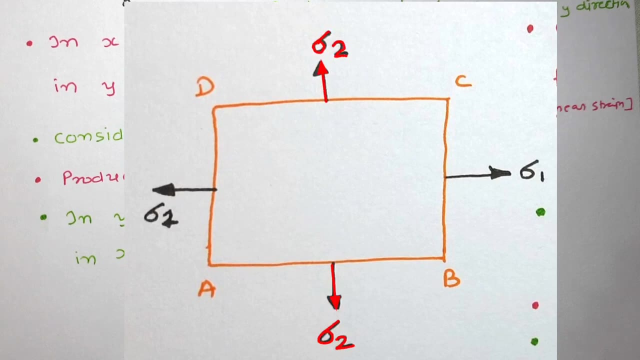 can write minus mu into sigma 1 upon e. so now let us see the stress produced by sigma 2 direction. in this figure we can see sigma 2 is acting in y direction. so in y direction there will be linear strain, and x direction it will be lateral strain. so sigma 2 will also produce strain in 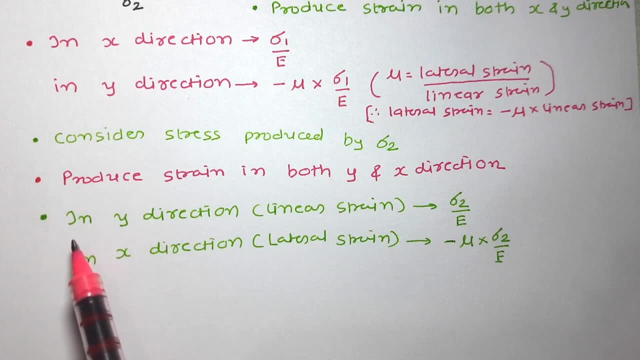 both the direction. so we can say: in y direction there will be linear strain that is equal to sigma 2 upon e and in average a direction there will be lateral strain that is equal to minus Poisson's ratio mu into linear strain, that is Sigma 2 by E. this value let epsilon 1, that is equal. 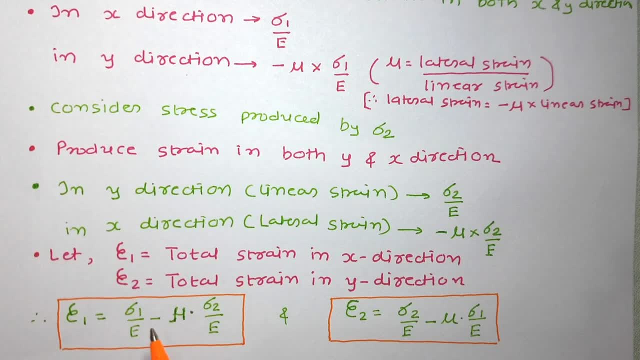 to total strain in X direction and epsilon 2, that is total strain in Y direction. so we can get summation of strain in X direction and Y direction. so in X direction the strain due to epsilon 1 is epsilon upon E and that is due to. 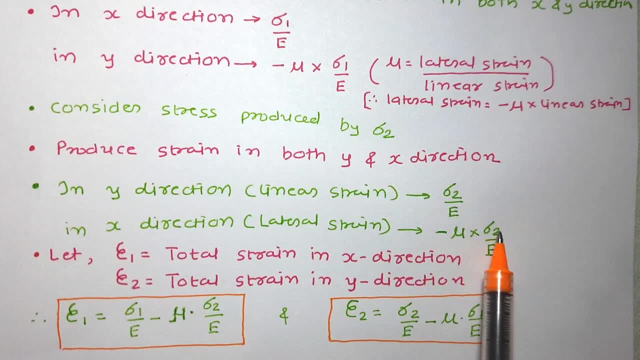 Sigma 2, that is minus Sigma 2 upon E. so we can get summation of this both terms right. so it will be Sigma 1 upon E minus mu into Sigma 2 upon E, and same way epsilon 2, that is total strain in Y. 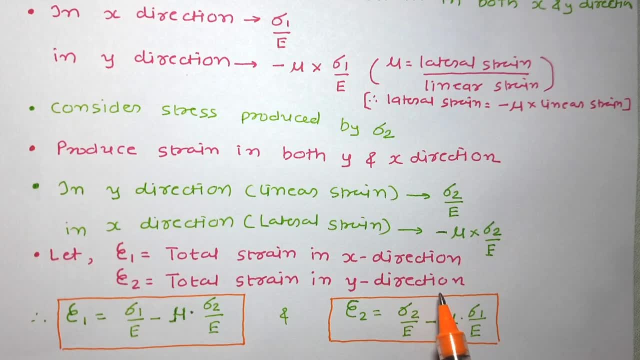 direction. so here we will take summation of both: stress in Y direction, so strain in Y direction. due to Sigma 2, that is Sigma 2 upon E, and due to Sigma 1, that is minus mu, into Sigma 1 upon E, so summation of this two. 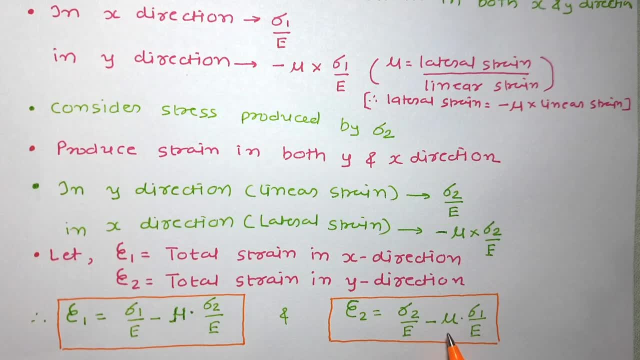 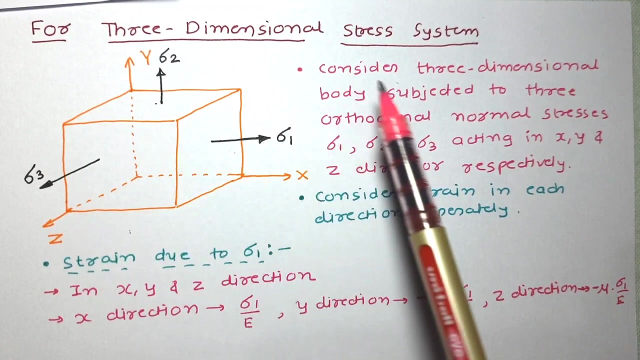 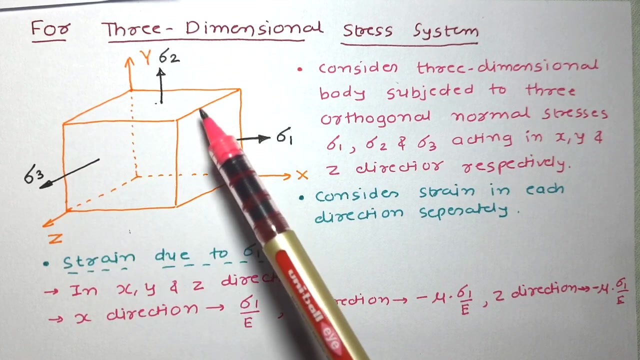 that will be Sigma 2 upon E minus mu into Sigma 1 upon E. so this is the relationship between stress and strain in two-dimensional system. so let us try to understand three-dimensional system in the figure. the figure consider a body which is three dimensional body and it is subjected to. 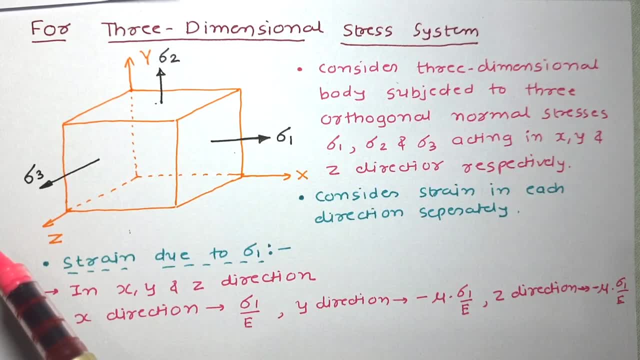 three-dimensional system with two-dimensional structure and three-dimensional area: orthogonal normal stresses: sigma 1 in x direction, sigma 2 in y direction and sigma 3 in z direction. now we will try to understand the strain produced by each stresses, in all direction and separately. so let us start with strain due to sigma 1. so sigma 1 is acting linear strain in x direction. 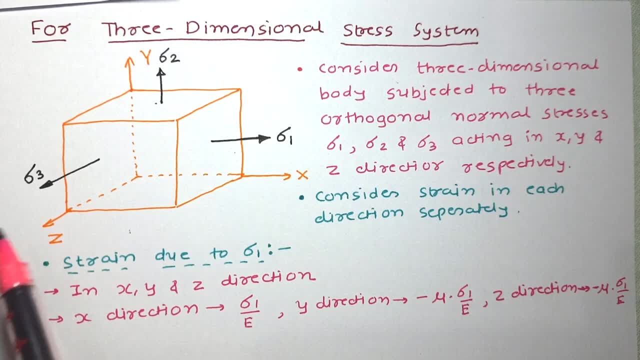 and lateral strain in y and z direction. so in x direction strain will be equal to sigma 1 upon e. in y direction it will be minus sigma 1 upon e into mu, that is lateral strain, due to sigma 1, that is poison ratio, into linear strain. so sigma 1 into e and same way in z direction it will be equal to minus. 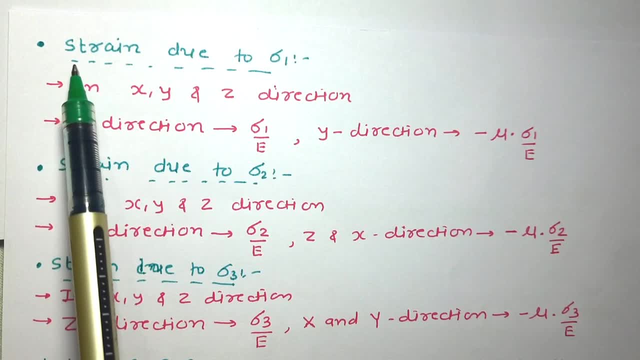 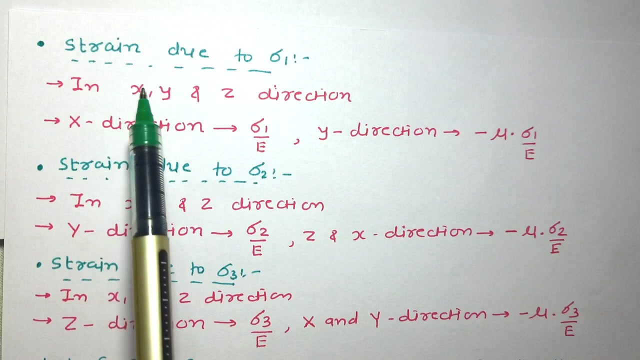 sigma 1 into e. now let us try to understand strain due to stress sigma 1. so sigma 1 is acting in x direction, but it effect will be in x, y and z, in all three direction, in x direction, where in x direction it will produce. 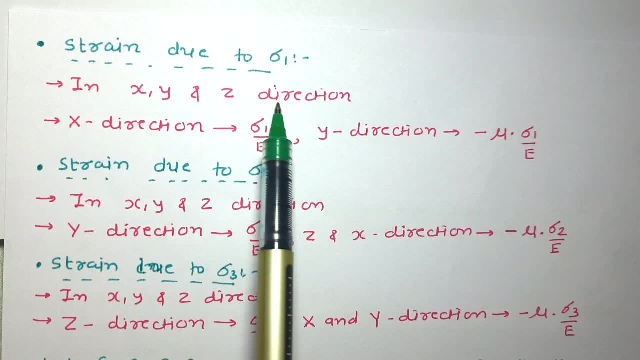 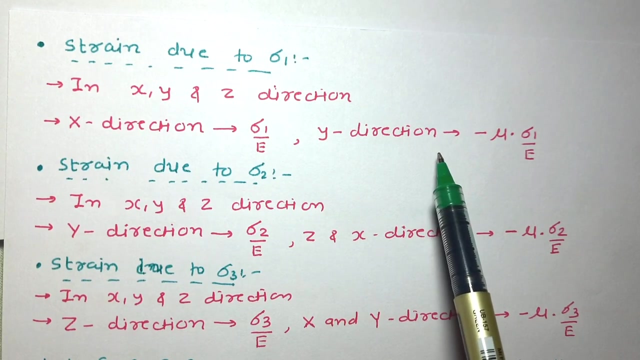 linear strain and in y and z direction it will produce lateral strain, so in x direction produce stress by sigma 1, so in x direction strain produced by stress, sigma 1, that is sigma 1 upon e, which is linear strain, and in y direction it will produce lateral strain, so will multiply linear. 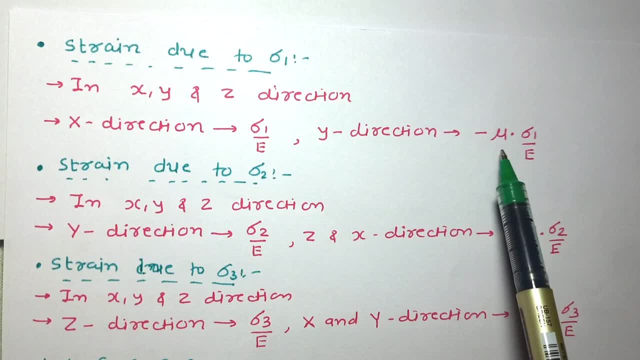 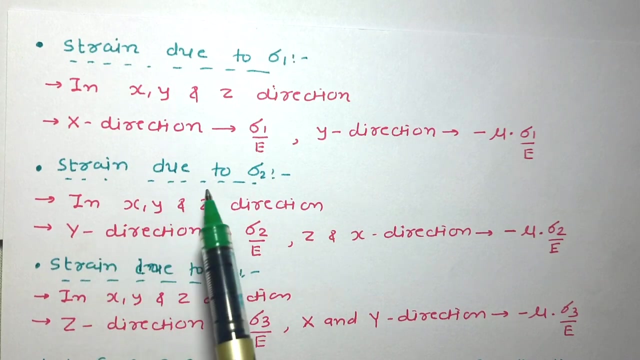 strain with modulus. so will multiply linear strain with poisons ratio. so this will lateral strain due to sigma 1, now stress produced by sigma 2, so it will also produce stress in all three direction. in y direction it will produce linear strain, that is sigma 2 upon e, and this stress, sigma 2 will 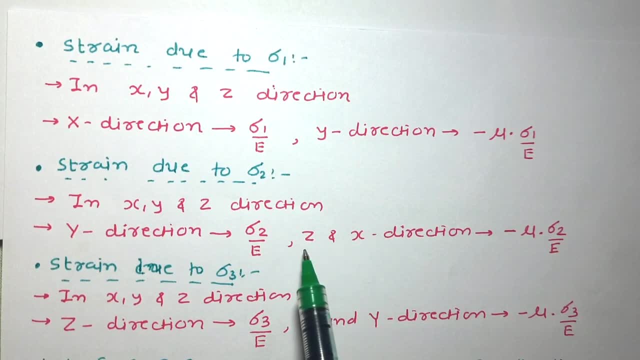 produce lateral strain in x and z direction, that is, minus Sigma 2 into E. the same way, strain produced by stress, sigma 3 will be in all three direction, but in Zed direction it will produce linear strain, that is, sigma 3 upon E, and in X and Y direction it will produce lateral strain that is equal to poisonous disorder. 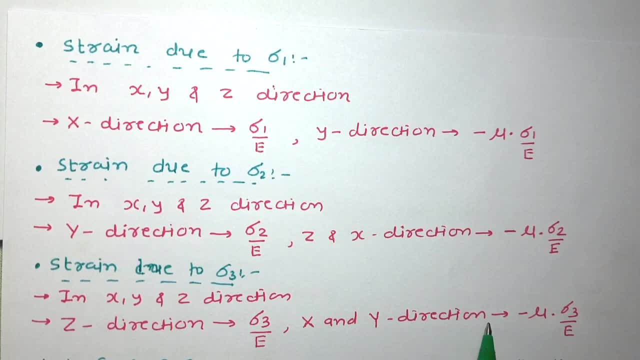 Soiteral strain is a positive, which means that at X, In X and Y direction it will produce integral strain, is equal to liners strain, that is, And if x and z are introduced to positive direction, then it will produce pag pasta with polar alpha. 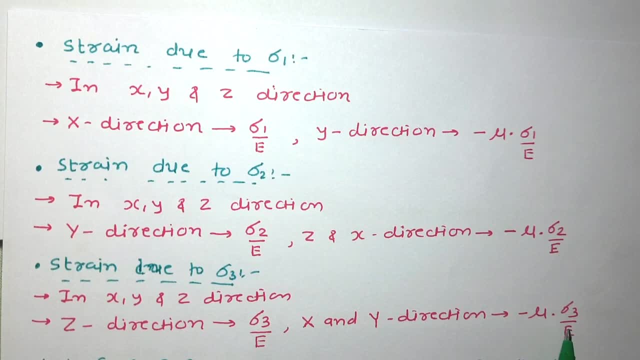 So if x and y are introduced to positive bastante, then it has negative pole and small. so if x, individual and small, will not be positive with polar alpha, then it will produce lateral strain, that is linear strain, as well as small strain that is equal to Poisson's ratio into linear strain, that is minus mu, into sigma 3 upon. 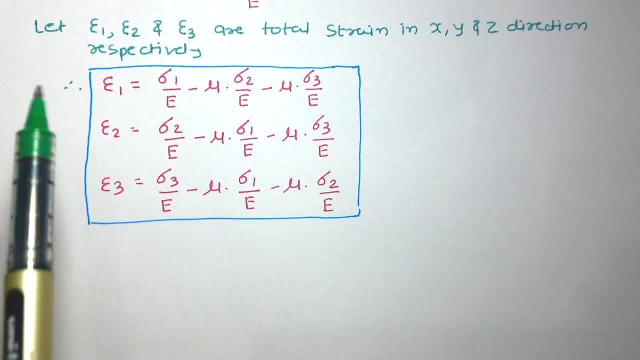 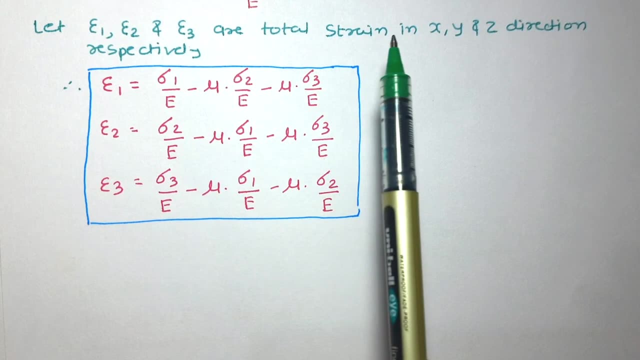 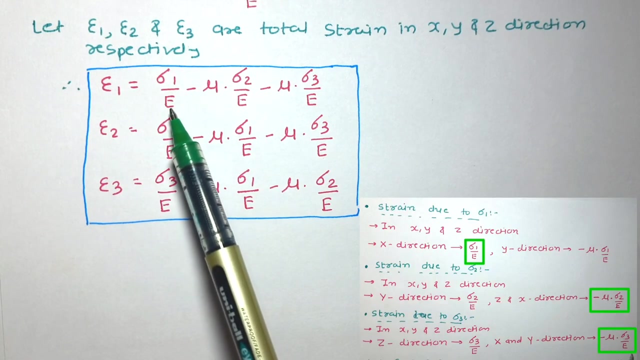 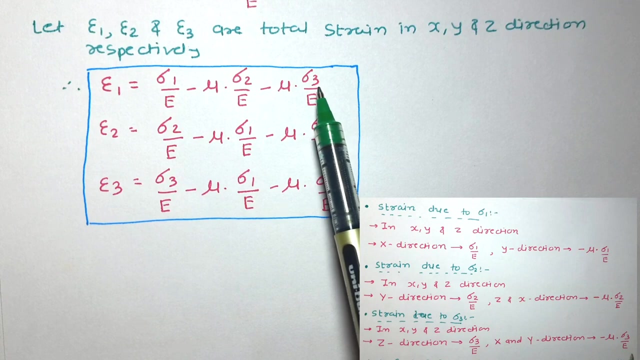 E. So now let epsilon 1, epsilon 2 and epsilon 3 are total strain in x, y and z direction respectively. So epsilon 1, that is equal to sigma 1 upon E. that is linear strain due to sigma 1 and lateral strain due to sigma 2 and sigma 3.. So it will be minus mu into sigma. 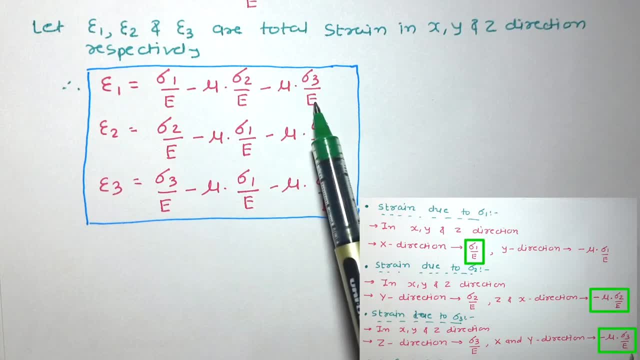 2 by E minus mu into sigma 3 by E. Same way for y direction. epsilon 2 is equal to sigma 2 upon E. that is linear strain, minus mu into sigma 1 upon epsilon. that is lateral strain due to sigma 1 and minus sigma 3 upon E. 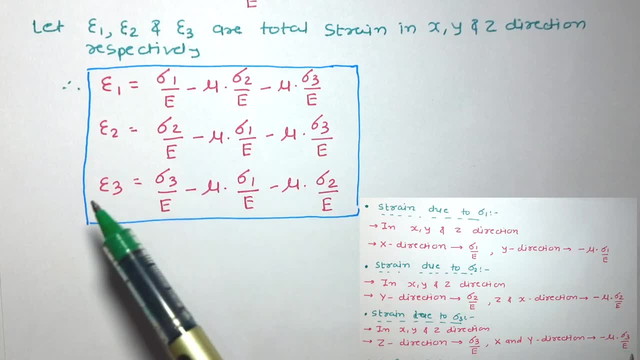 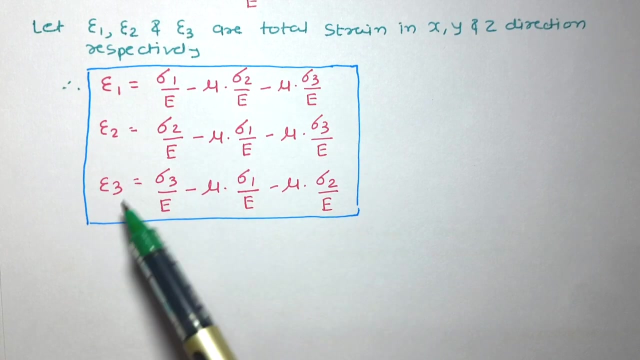 That is lateral strain due to sigma 3, and in z direction it will be sigma 3 upon E. that is linear strain due to sigma 3 and lateral strain due to sigma 1 and sigma 2, with minus sign, so minus sigma 1 upon E, minus mu, into sigma 2 upon E. So this way we can work out. 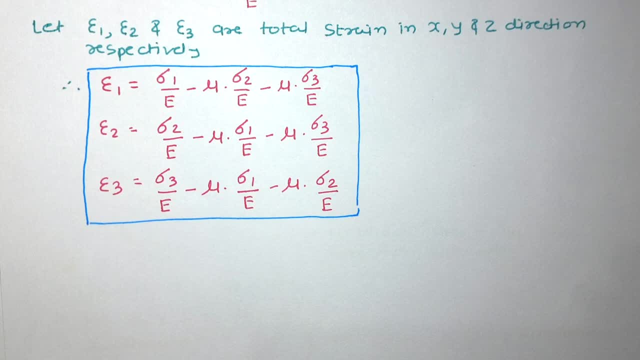 in three dimensional system. Thank you for watching this video. If you have any doubt or any query, please write in comment box. Thank you, Thank you very much.